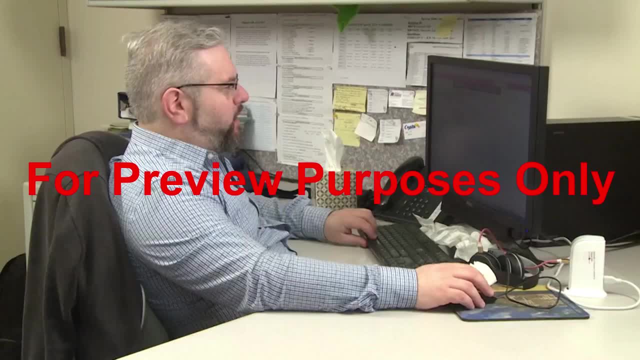 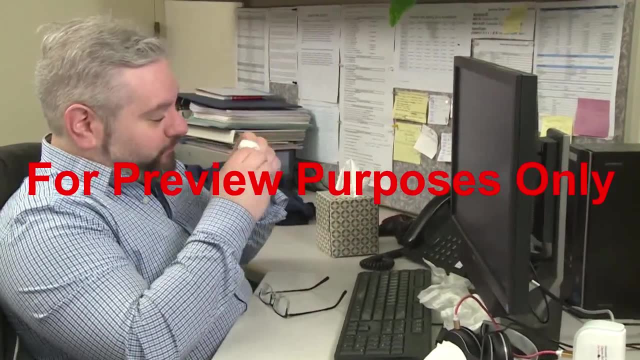 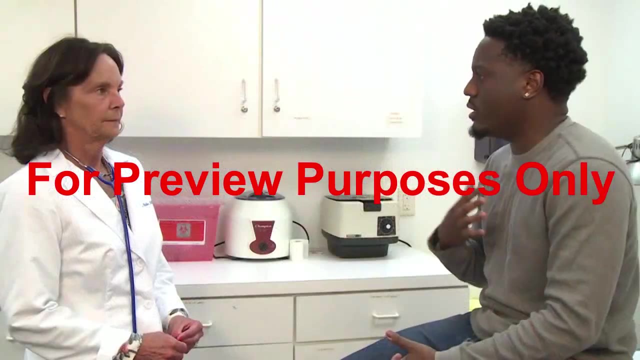 such as asthma and emphysema. Different people can react to bad air in different ways, but any of these symptoms could indicate that there is a problem with the air in your building, Especially if you experience them repeatedly, When a person's health problems can be directly linked to poor air quality in a building. 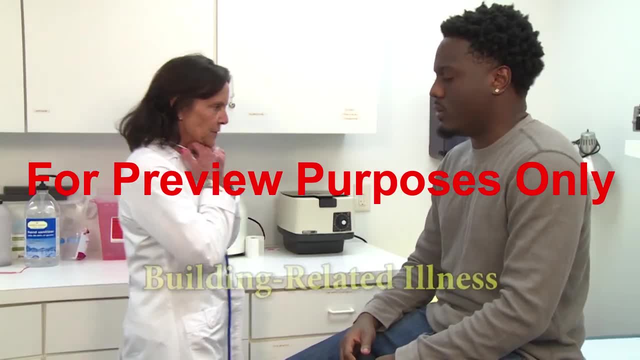 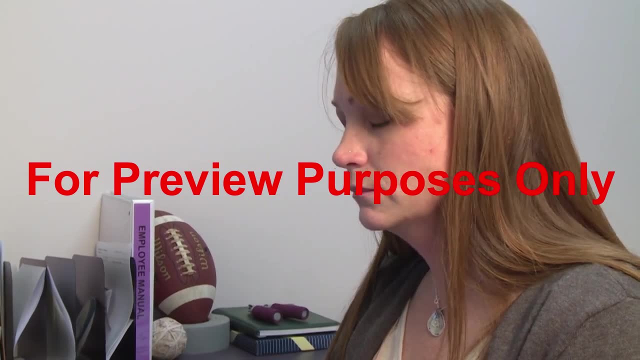 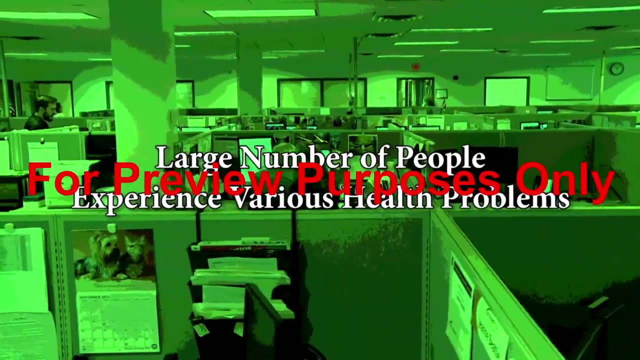 that set of symptoms they are experiencing is called a building-related illness. But identifying the cause of bad air can often be a challenge. You may have heard of a condition known as sick building syndrome. This occurs when a large number of people in a building experience. various health problems. You may have heard of a condition known as sick building syndrome. This occurs when a large number of people in a building experience various health problems. You may have heard of a condition known as sick building syndrome. This occurs when a large number of people in a building experience various health problems. 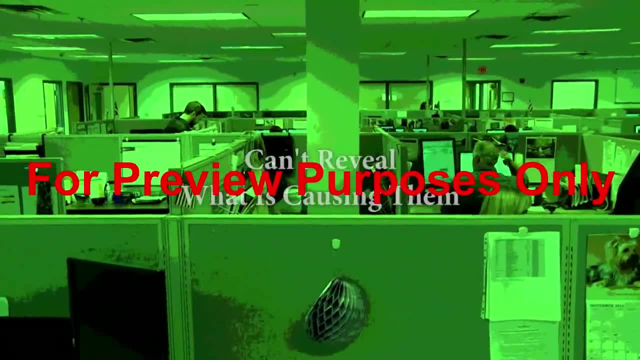 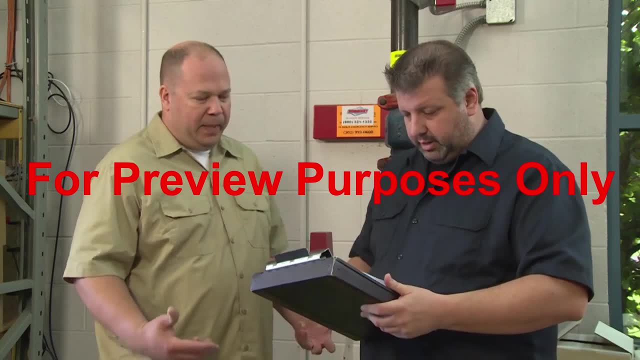 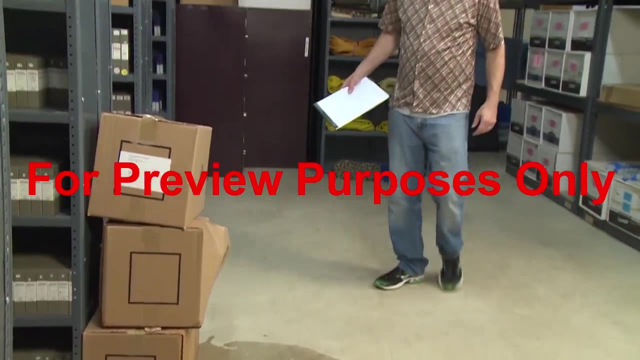 Their symptoms disappear when they leave the building, But even a professional air quality investigation can't reveal what is causing them. Something in the building seems to be the culprit. However, what that thing is can be a mystery. But even if the cause of the bad air can be identified, this is only the beginning of 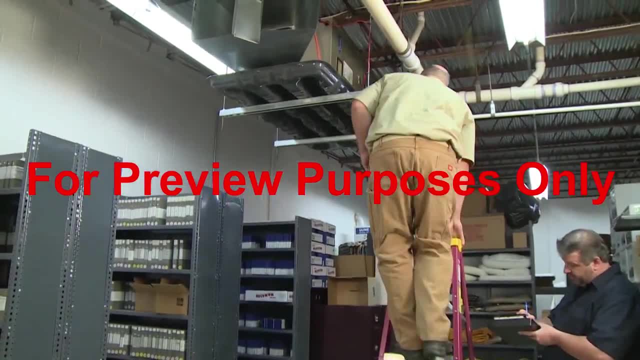 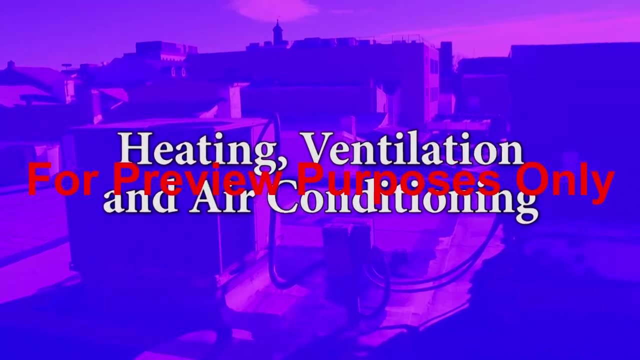 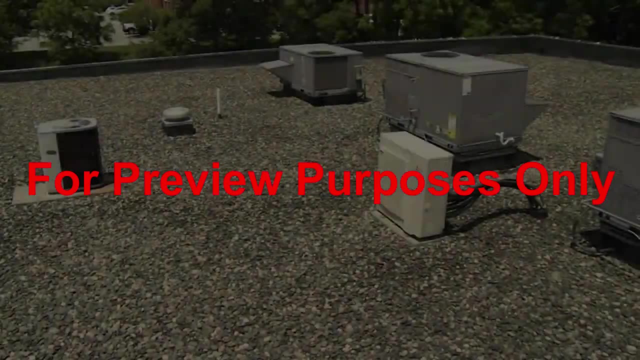 dealing with it. The problem must be corrected and prevented from occurring again in the future. You might see something like this before Take care of the building in the future. The three main factors that affect the quality of indoor air include the building's HVAC system. 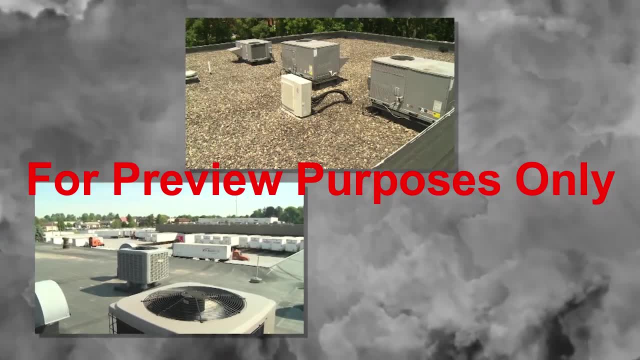 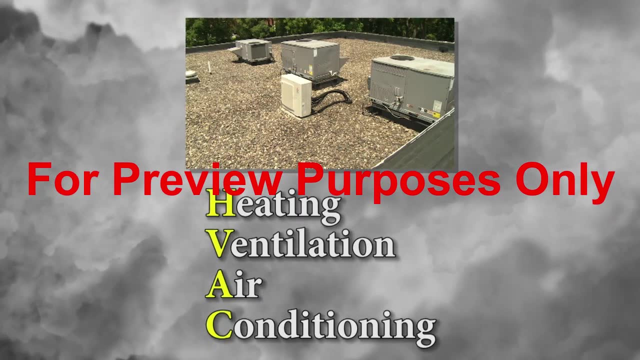 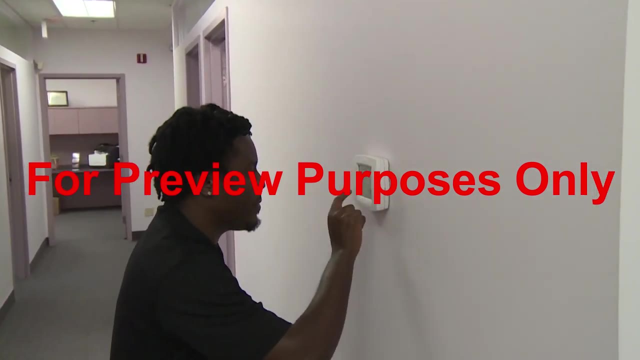 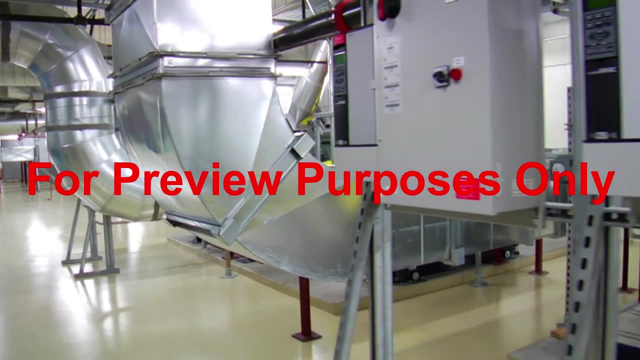 sources of contamination, both inside and outside the building and the people who occupy the building. HVAC stands for Heating, Ventilation and Air Conditioning. An HVAC system controls the temperature, humidity and circulation of air throughout a facility, Depending on the building's size and the activities that go on inside it. the system 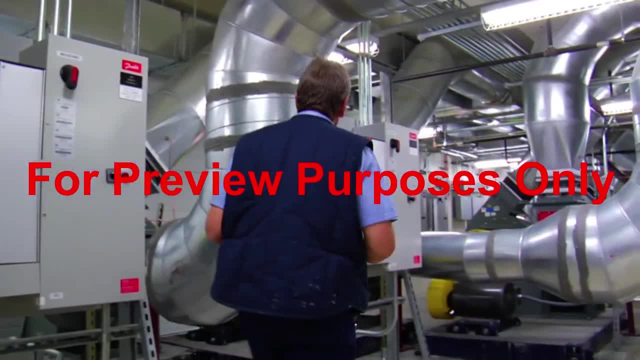 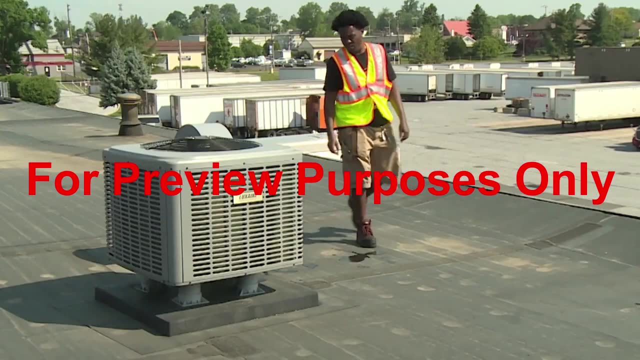 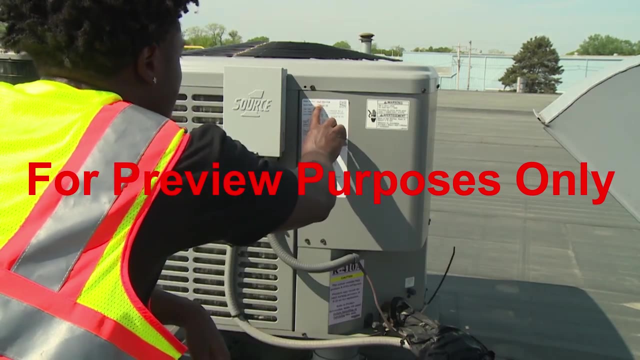 can be fairly complicated. To do its job correctly, the system must be customized for the facility and balanced for the different areas within it. Problems with the design or operation of an HVAC system can significantly affect the quality of the air that is delivered to the occupants of the building. 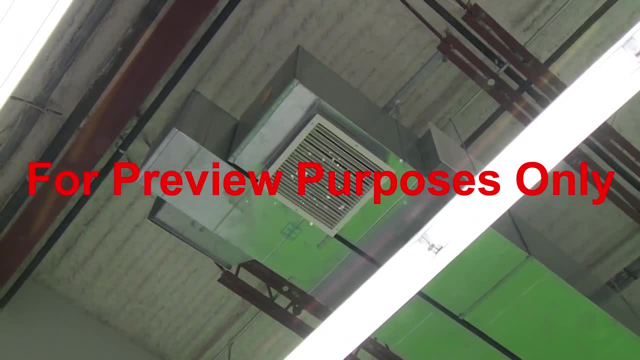 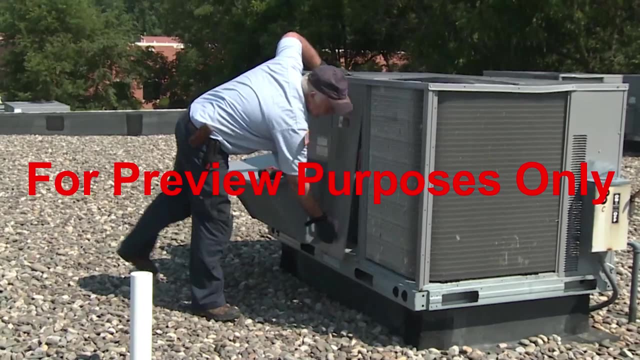 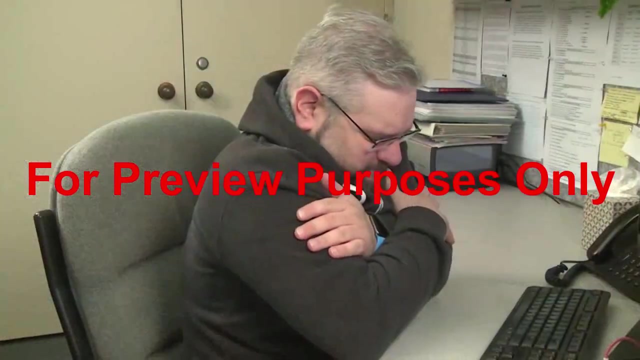 For example, if a system does not filter the air correctly or its filters become dirty or clogged, the system could actually spread contaminants throughout the facility. Regular inspections of the system, including its filters, can prevent this and other problems. What you do can also affect how well the HVAC in your building works too. 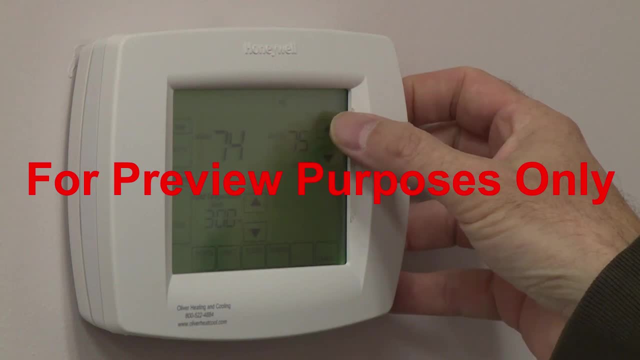 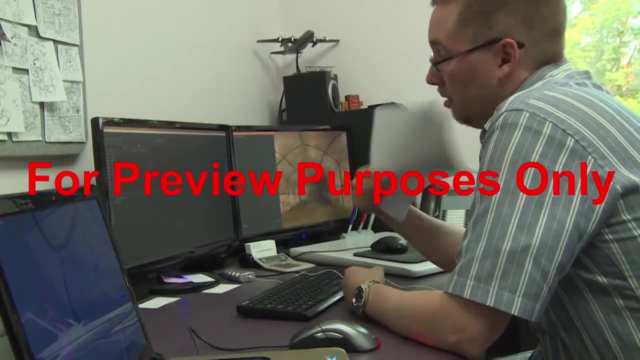 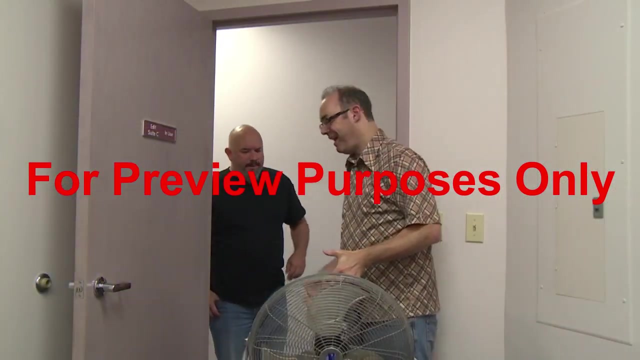 Changing a thermostat setting, for example, may make you more comfortable, but it can disturb the balance of the system, which could cause trouble for others. So you should leave thermostats alone unless you have been authorized to adjust them. Other fixes like adding fans to your work area or blocking air vents can affect the 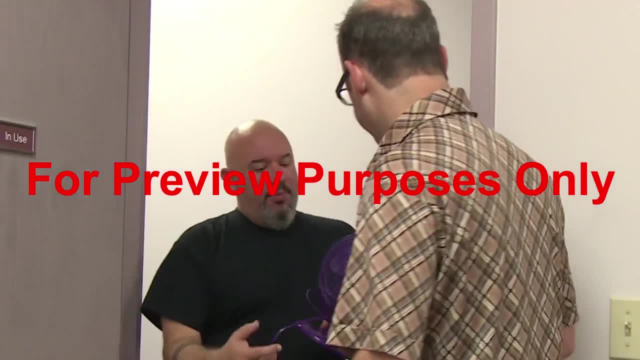 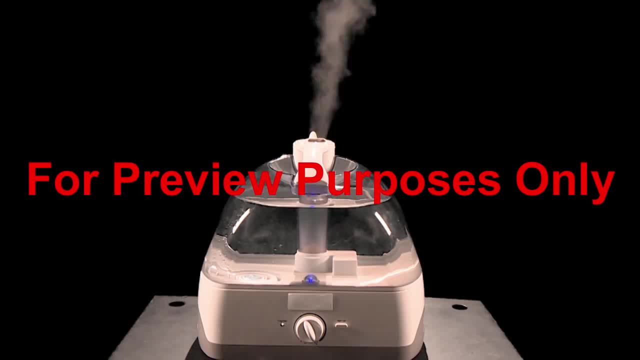 way, the HVAC functions as well, So you shouldn't make these types of changes without first consulting your supervisor. While humidifiers and dehumidifiers can help to control the amount of air that is delivered, you should check with your supervisor before using them too. 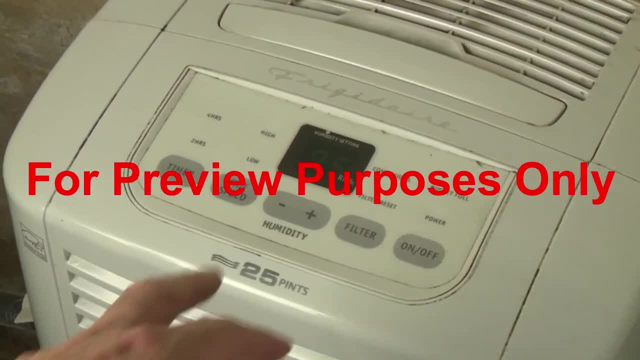 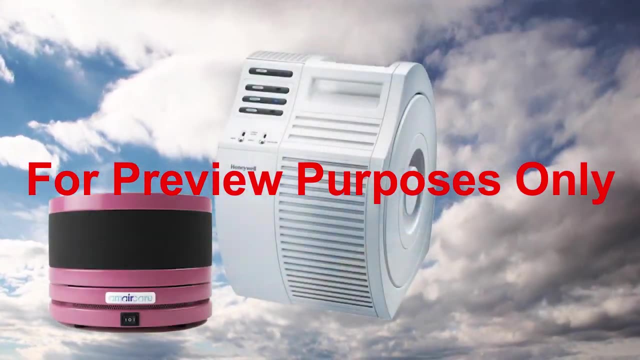 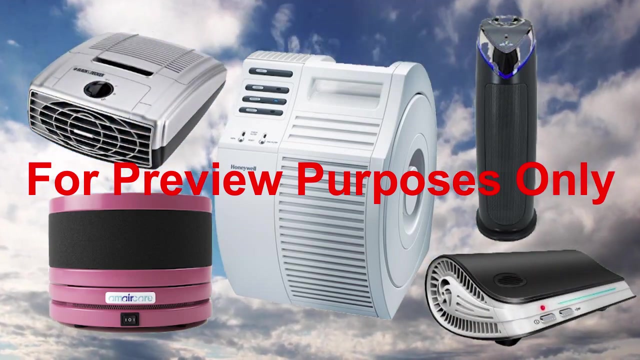 They can conflict with your facility's HVAC or possibly damage equipment or materials in the facility. The same goes for portable air cleaners and ionizers. They can be effective for removing dust and other contaminants from indoor air, but could cause other problems. If you are permitted to use these types of devices, remember to clean their filters. 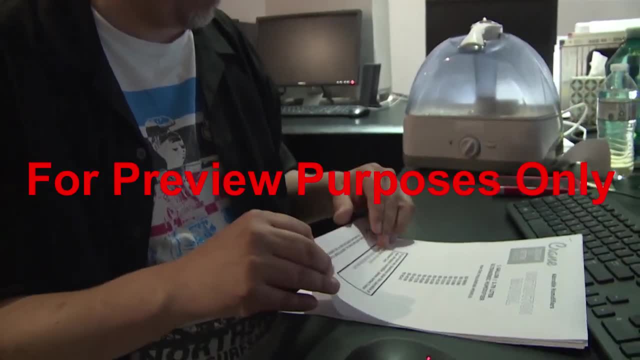 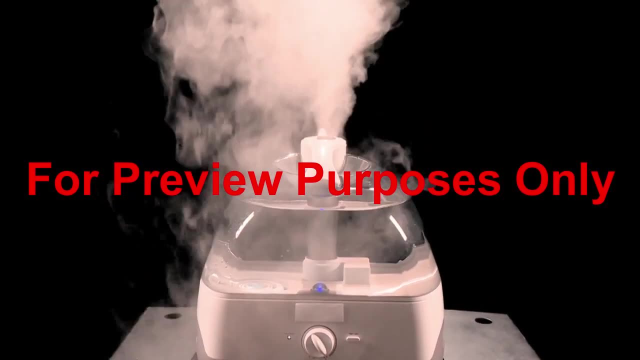 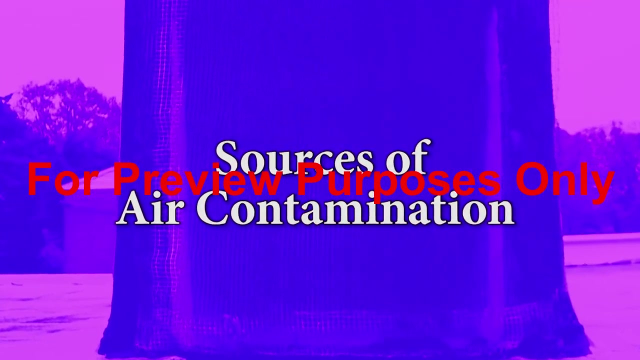 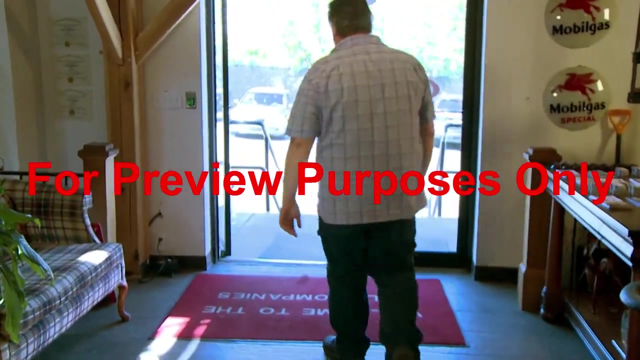 reservoirs and drip pans And always follow the manufacturer's instructions for servicing them. Without regular maintenance, they can make the air quality worse instead of better. To keep the air in a building healthy, any sources of contamination, either inside or outside of the structure, 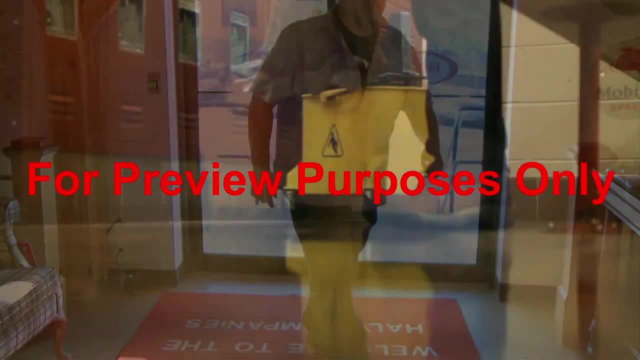 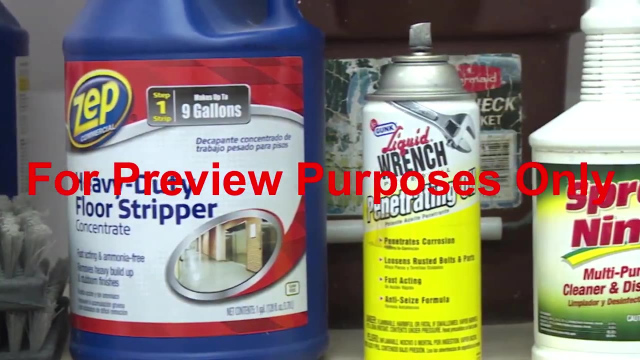 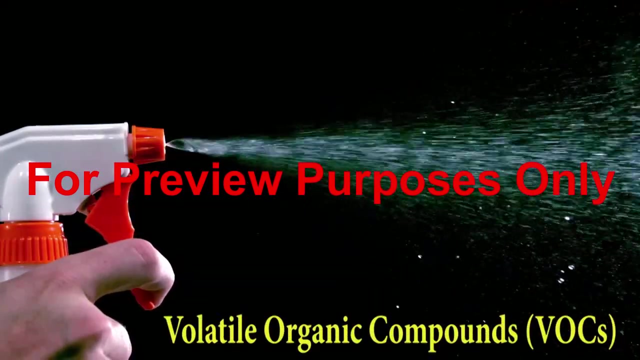 must be identified, then eliminated or controlled. For instance, a variety of cleaning products are used in most buildings. Adhesives, solvents and other chemicals may also be present. These can release volatile organic compounds, VOCs- into the air. 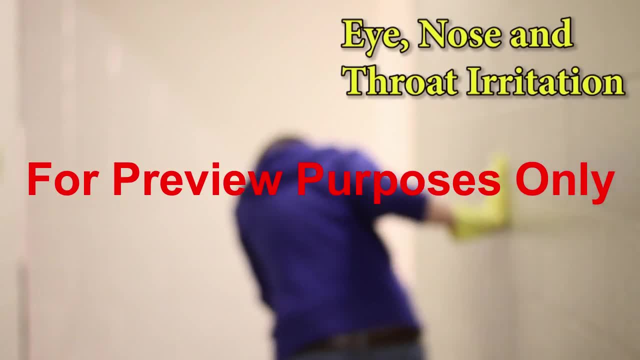 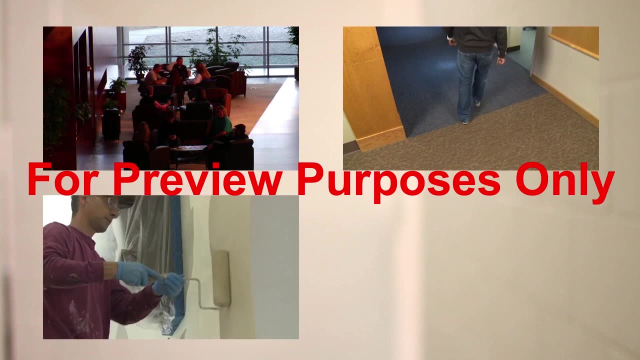 The health effects of VOCs can range from eye, nose and throat irritation to liver and kidney damage, possibly even cancer. Furniture, carpeting, paint and sunscreens can also be used to clean the air. For example, if you have a problem with the air quality of your building, you should 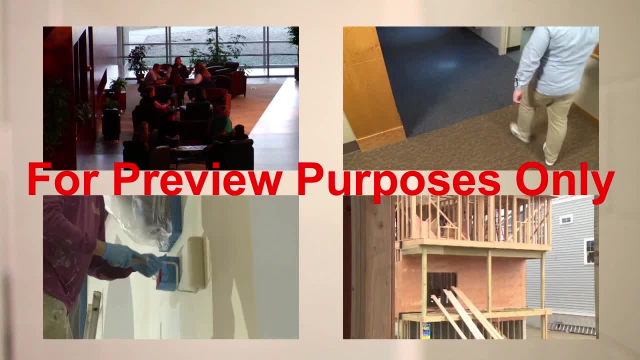 go to a fire- Sax-ாy sá hi 용, spray it and mark the windows. These'll probably haия other environmental damages. Receiving aacy and some types of construction materials can release VOCs that were used in manufacturing them. 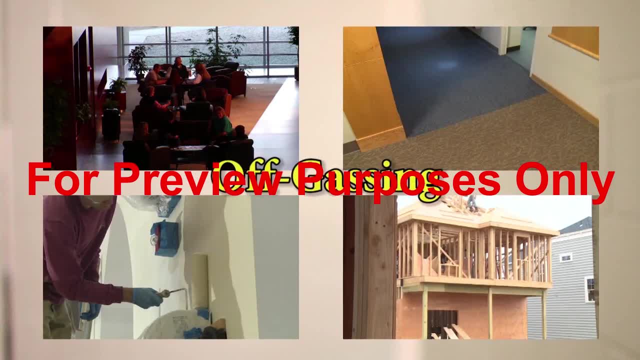 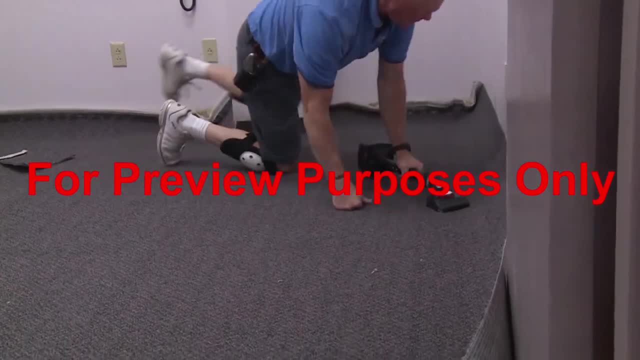 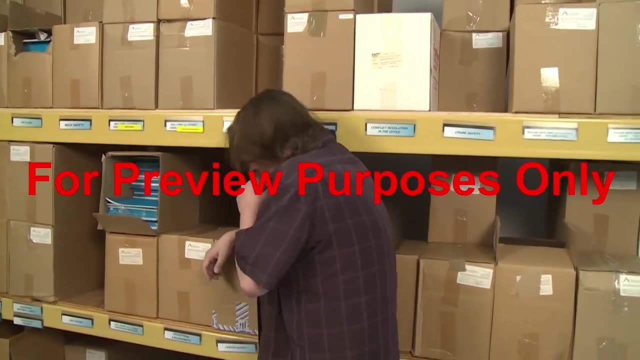 This process is known as off gassing. Off gassing can be especially severe in buildings that are new or recently remodeled or renovated. Another common indoor contaminant is dust. When it is stirred up into the air, dust can irritate the eyes, nose and throat, and not 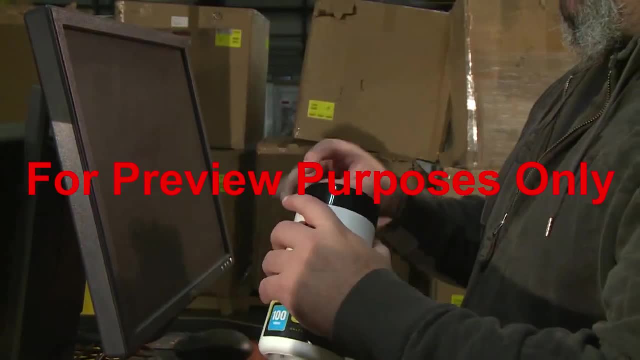 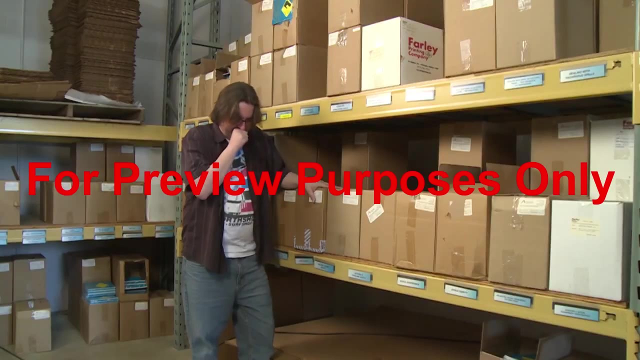 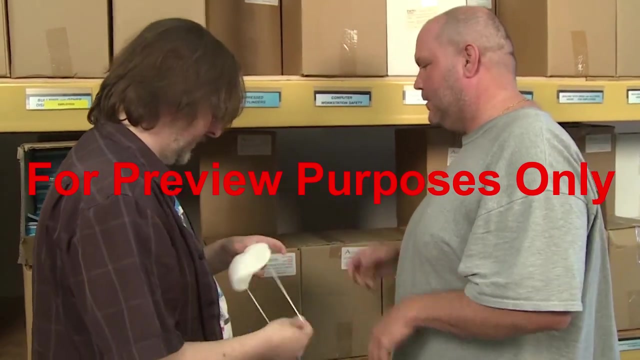 just for people who are allergic to it. A good way to reduce airborne dust is by wiping down surfaces regularly with a damp cloth or towel. If you work in an area or with a process that produces a lot of dust, you may want to talk to your supervisor about wearing a filter mask or other respiratory protection. 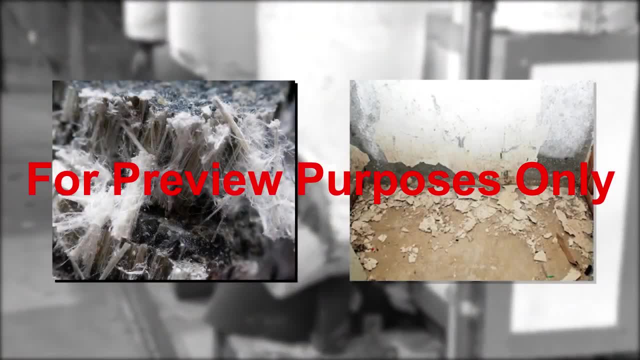 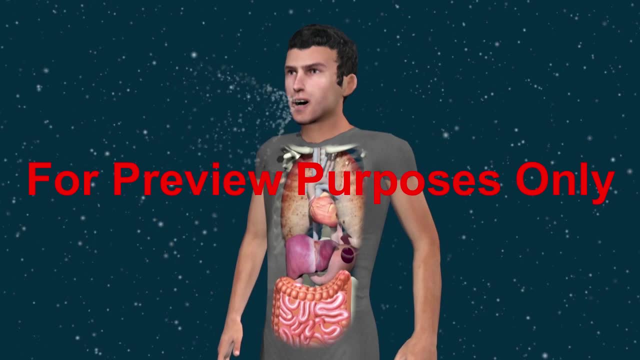 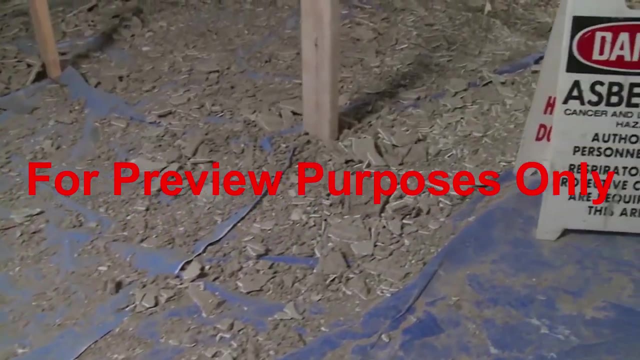 Asbestos fibers and lead dust are two especially hazardous substances that can be found inside some buildings. Inhaling either of these materials can lead to serious physical damage, disease and even death. Requirements for identifying, controlling and removing these contaminants in public and private buildings. 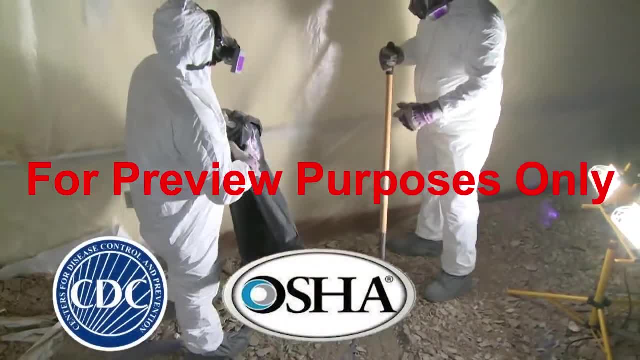 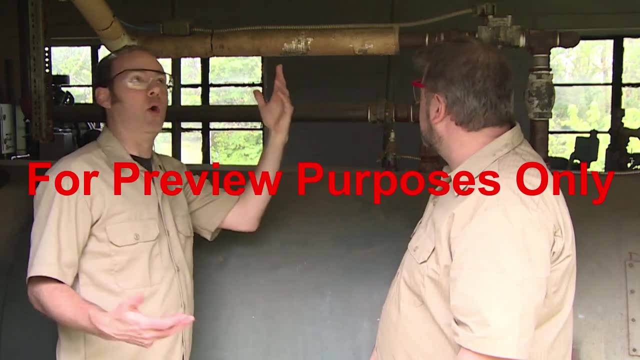 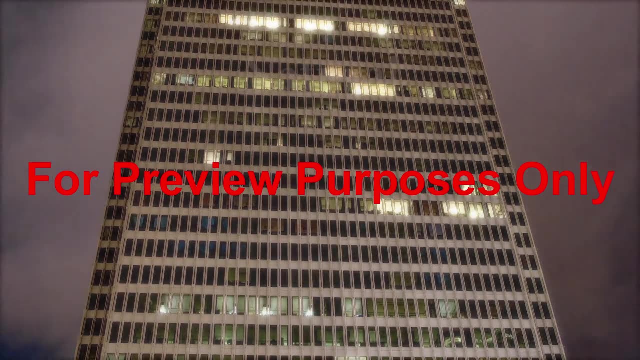 are strictly enforced by OSHA, the Centers for Disease Control and Prevention and the EPA. Your employer will tell you if there are any lead or asbestos hazards in your workplace. Air contaminants that can come in from outside your building include natural substances such as dust, pollen and fungi spores. 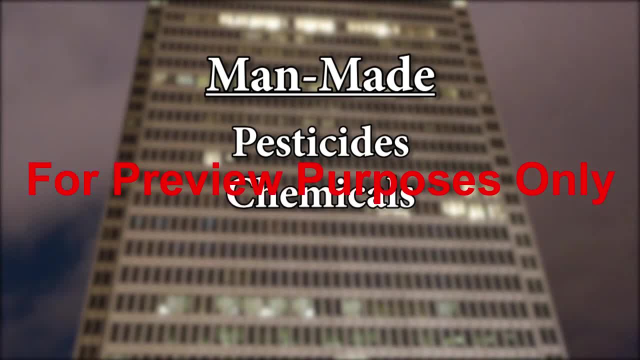 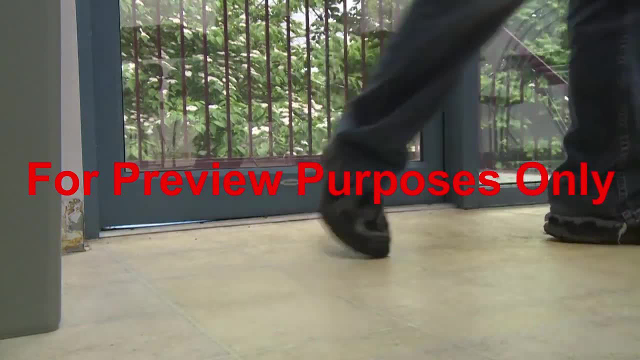 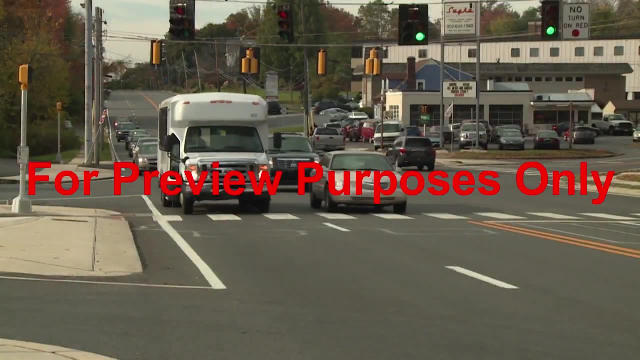 as well as man-made materials such as pesticides, chemicals and pollutant emissions. Outdoor contaminants like these can get inside through open doors or windows, or even the air intake vents of your building's HVAC. Carbon monoxide is a hazardous gas that can originate outside the building. 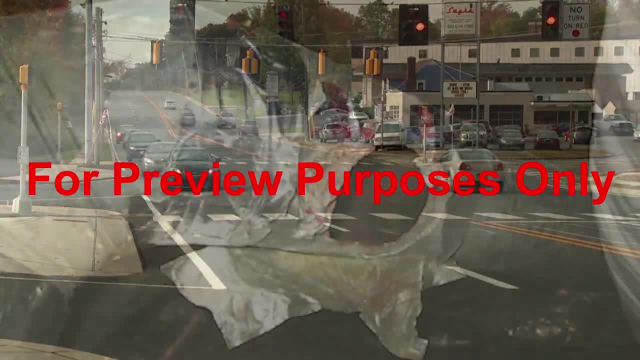 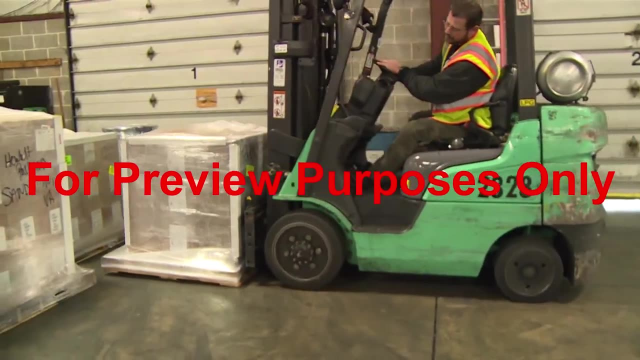 and exhaust emissions from cars, trucks and other vehicles, As well as inside from leaking furnaces, chimneys or flues, and from gas and propane or diesel-powered forklifts. Standing water can collect outside on rooftops in wet weather. 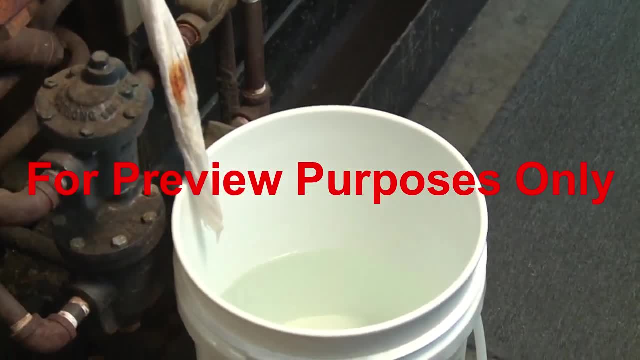 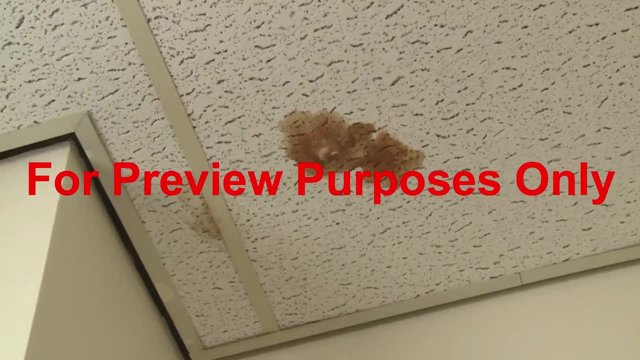 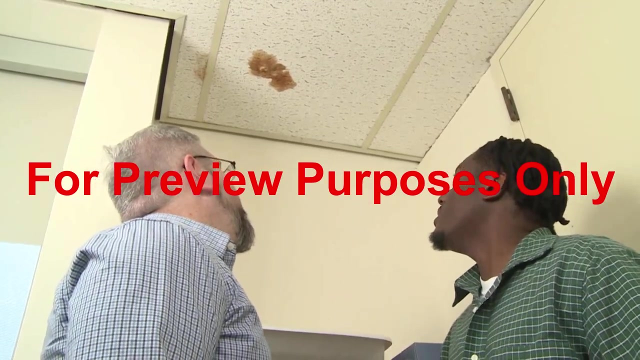 or inside from leaky pipes or other sources and provide a breeding ground for bacteria and mold. Water stains or other damage could indicate that this is happening in your building. If you see clues like these, notify your supervisor so the problem can be addressed. 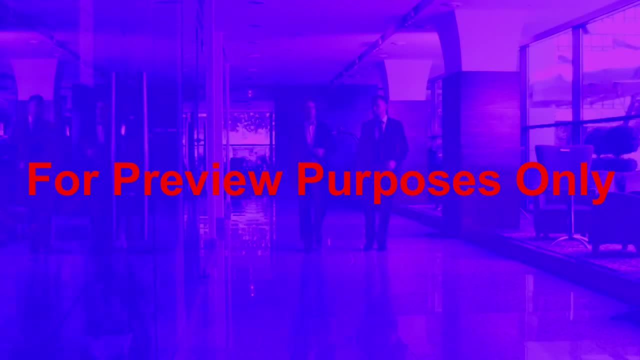 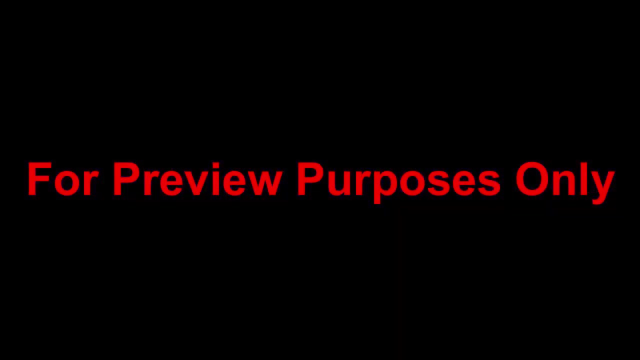 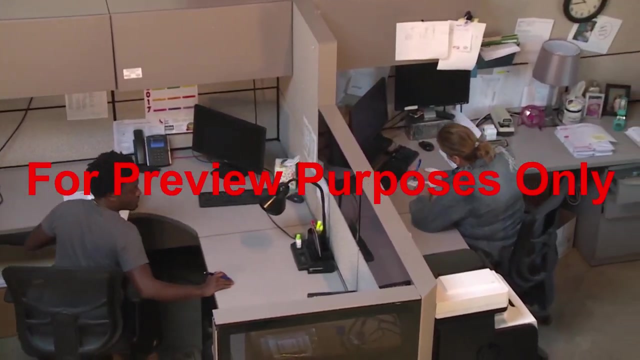 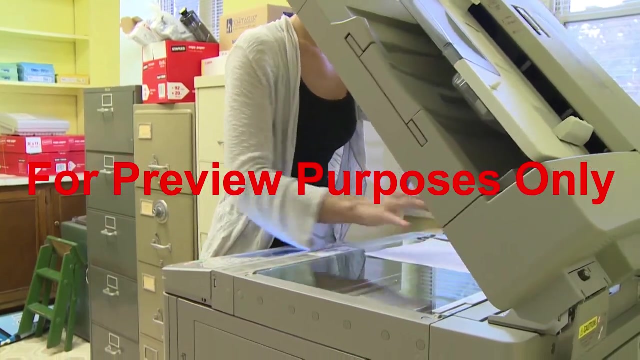 The third factor that can significantly affect indoor air quality is us, the people who work in a building. There are things that we can do and avoid doing that can significantly improve the quality of the air we breathe on the job. For example, leaving leftover food sitting around the door. 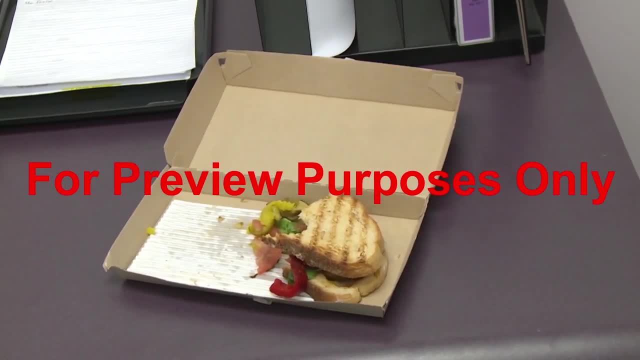 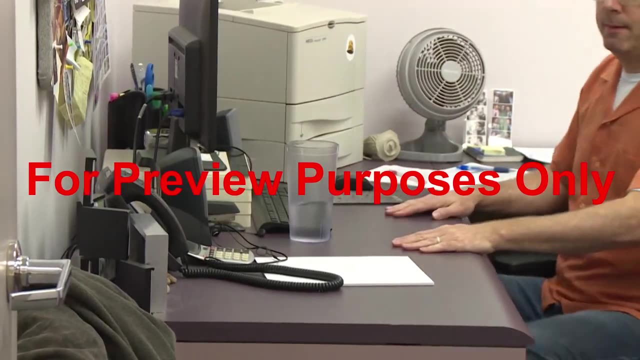 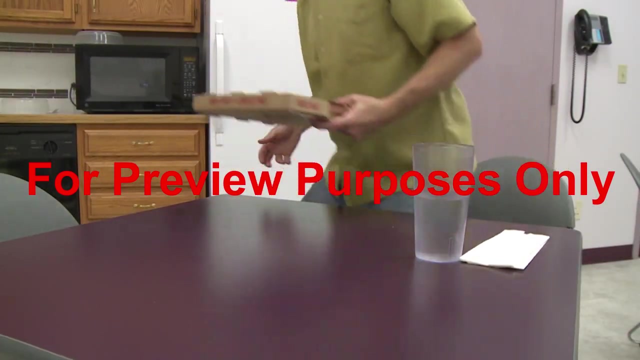 gives bacteria, mold and fungus a place to grow and flourish. Used soft drink, coffee and milk containers will do the same thing. Even a half-empty cup of water can become a source of contamination. You can prevent this by refrigerating or throwing away all leftovers. 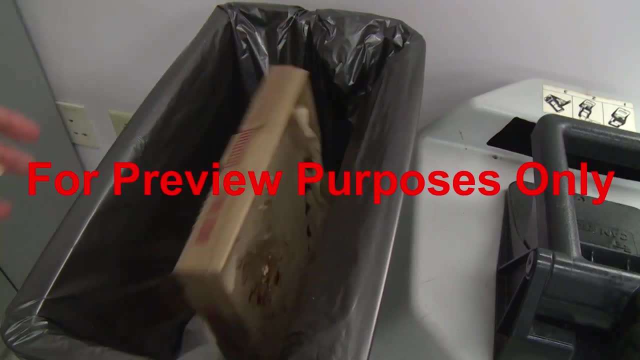 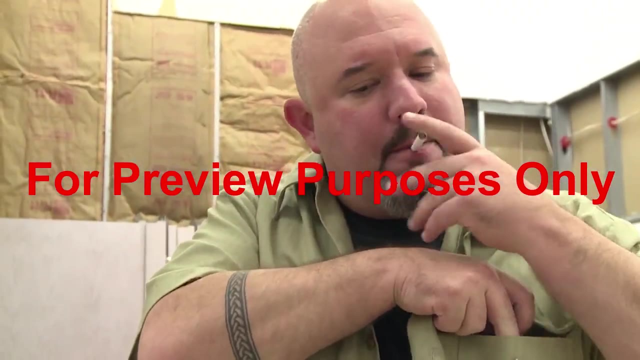 Bacteria, mold and fungus can also grow in trash, so make sure waste bins are emptied and cleaned on a regular basis. Tobacco smoke can be hazardous to everyone, smokers and non-smokers alike. To protect employees who don't smoke from the air contaminants, 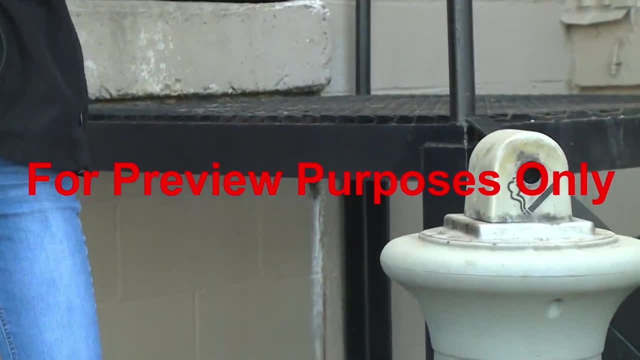 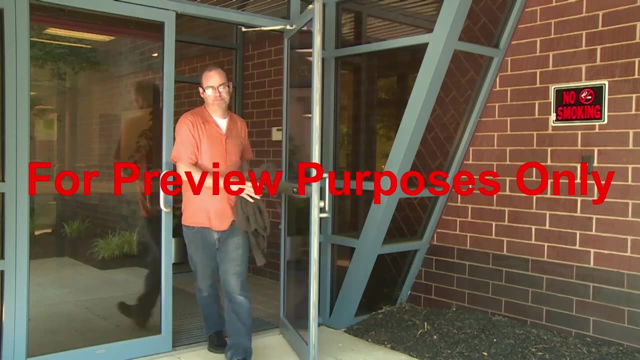 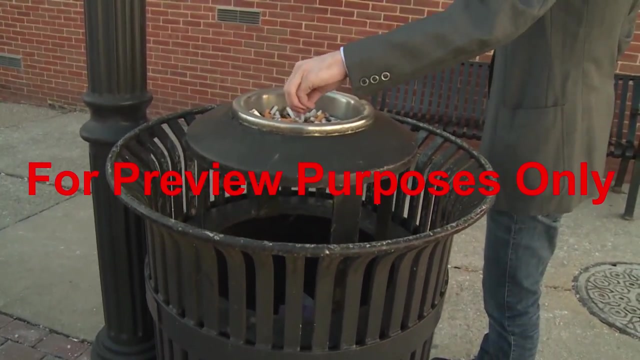 created by those who do. many employers have created dedicated smoking areas that are set apart from the rest of the facility or ban smoking in their facilities altogether. If you smoke, be sure to follow your facility's smoking policy and smoke only in designated areas. 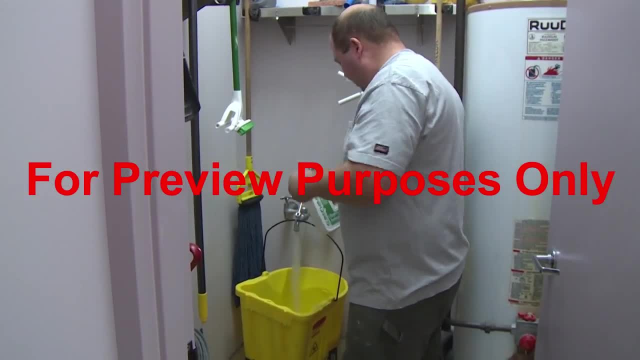 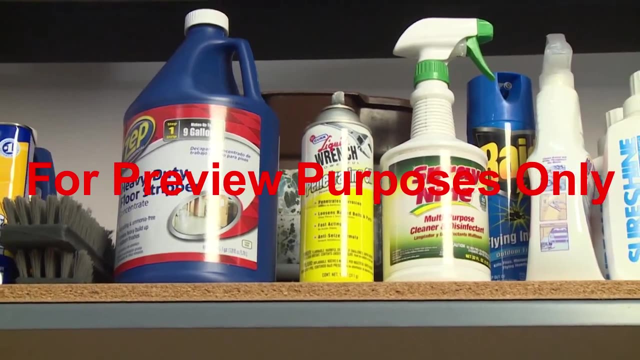 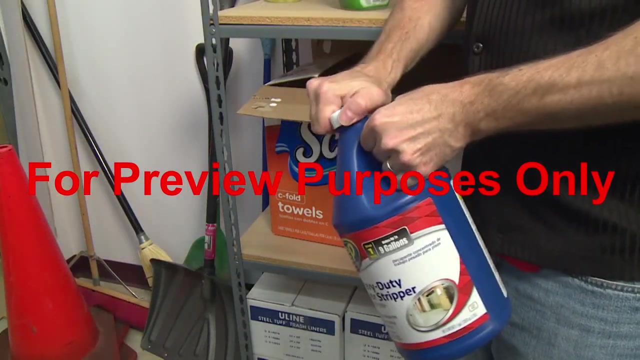 Earlier we mentioned that cleaning products, solvents and other chemicals can affect the quality of the air we breathe indoors. You can reduce their impact significantly by following safe housekeeping practices when you use them. Reseal cleaners and other chemical containers when they're not in use. 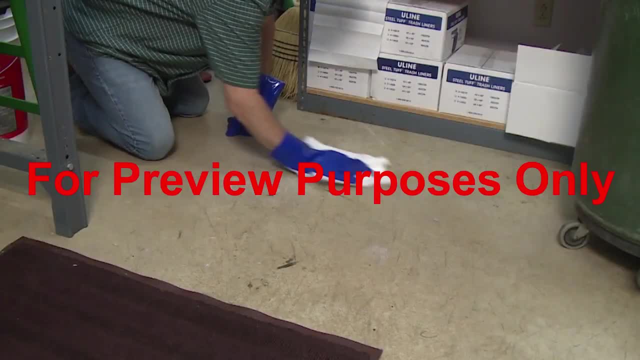 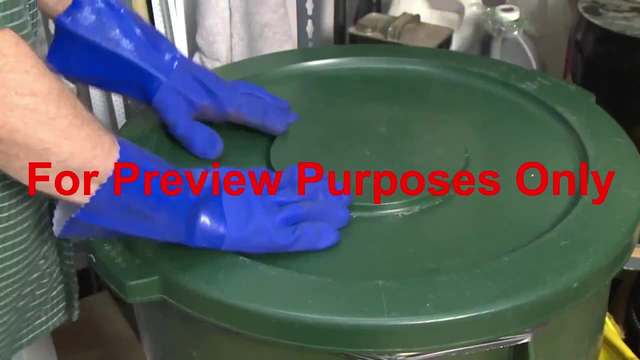 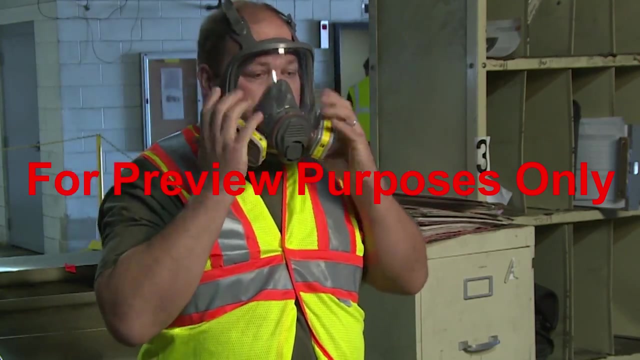 Store them properly, Clean up any leaks or spills immediately And place all contaminated rags, towels or other materials in a covered container or sealed bag. In some situations, extra ventilation or respiratory protection may be required to deal with these situations If you notice any potential sources of air contamination. 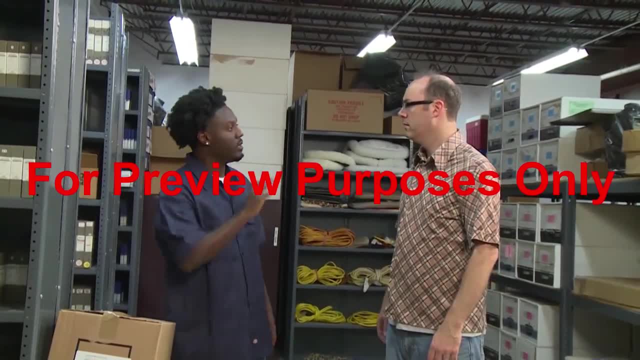 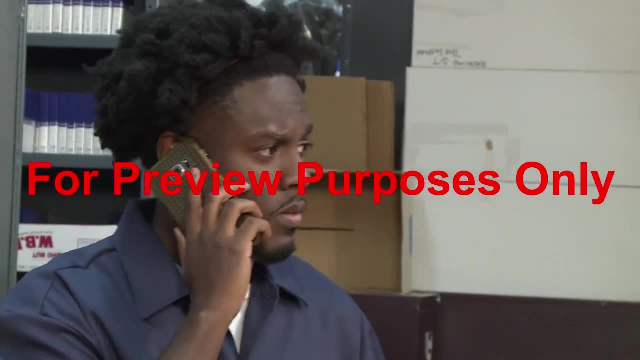 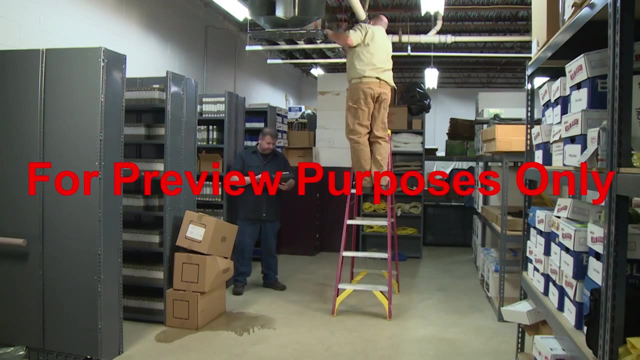 or other air quality problems in your workplace, you should notify your supervisor at once. If the problem is more than they or other staff members can handle, professionals will be called in to investigate the situation. In general, you should try to keep clear and let these people do their work.